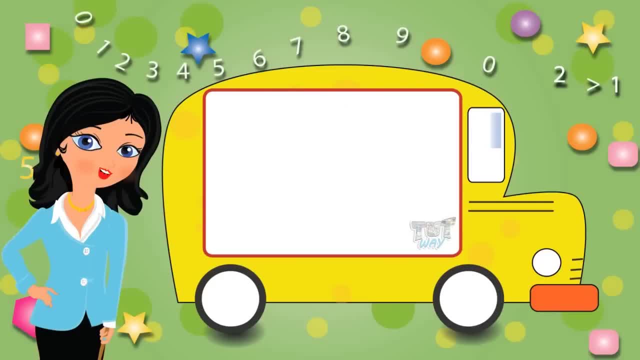 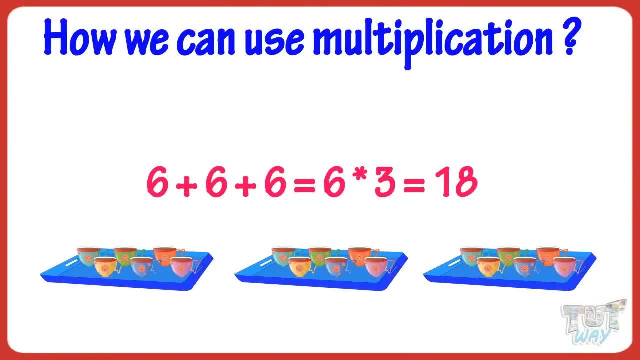 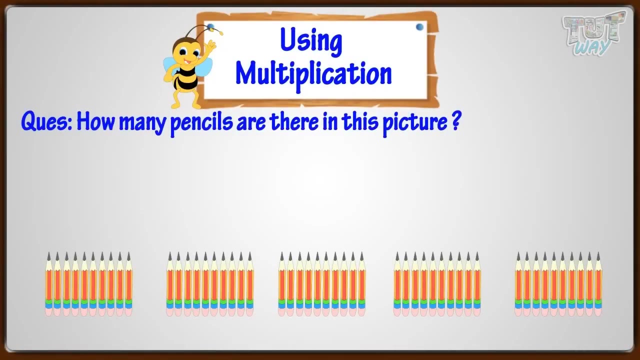 Hi kids, Today we will be learning how we can use multiplication in our problems. So let's start. Can you calculate how many pencils are there in this picture? 5 sets are there and 10 pencils are there in each set. So we need to add 10- 5 times. 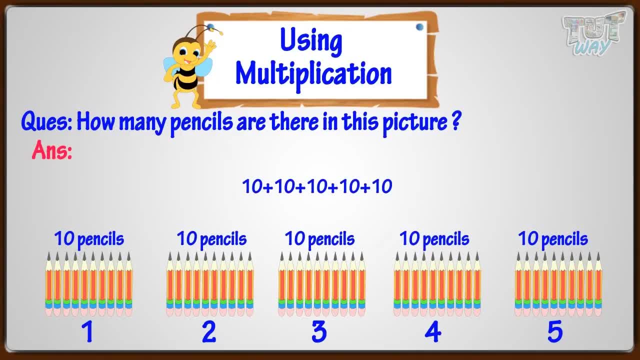 Remember, we use multiplication for repeated addition problems. So instead of adding 10 5 times, we can multiply 10 with 5. So we get. So there are 50 pencils in the picture, Isn't it easier? 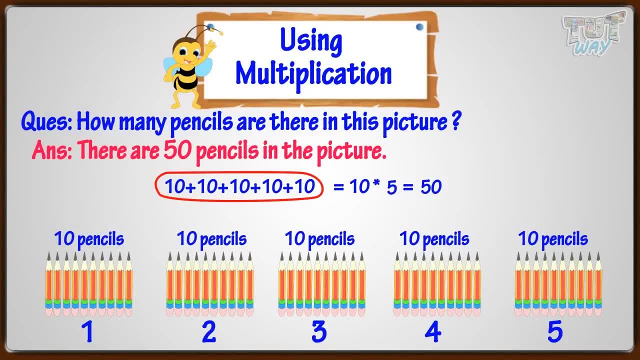 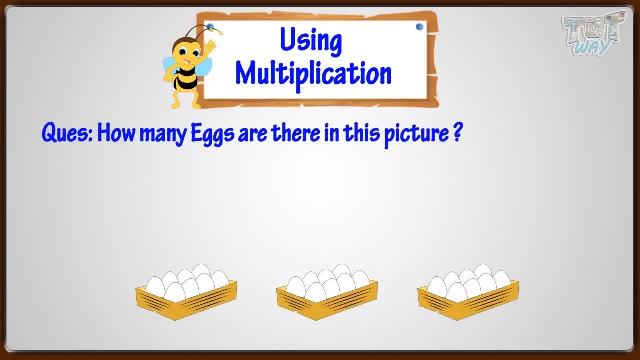 Let's take one more example. Can you calculate how many eggs are there in this picture? 3 trays are there and each tray has 8 eggs. So we need to add 8 3 times. Remember We use multiplication for repeated addition problems. 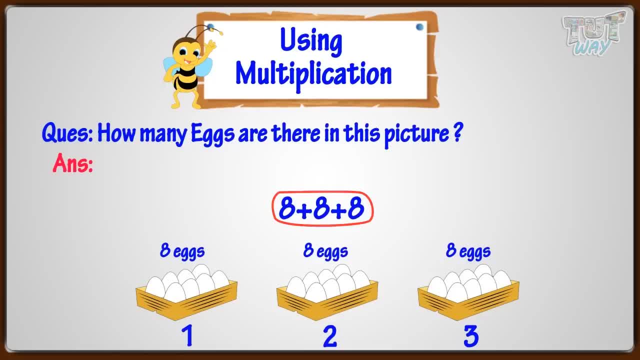 So instead of adding 8 3 times, we can multiply 8 with 3. So we get 24.. So there are 24 eggs in the picture. Isn't it easier? So let's take one more example. 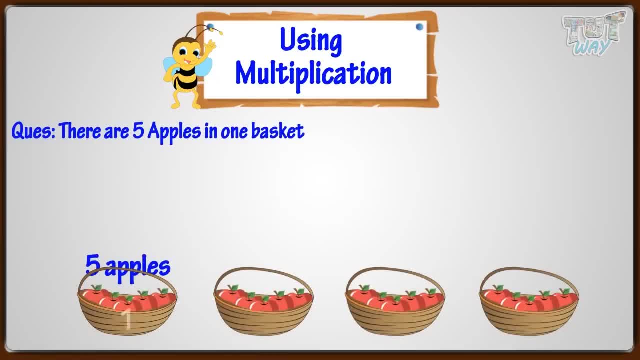 There are 5 apples in one basket, Then 4 baskets will have. how many apples You need to add 5, 4 times here And you now know You can write repeated addition in the form of multiplication sentence. So 5 plus 5 plus 5.. 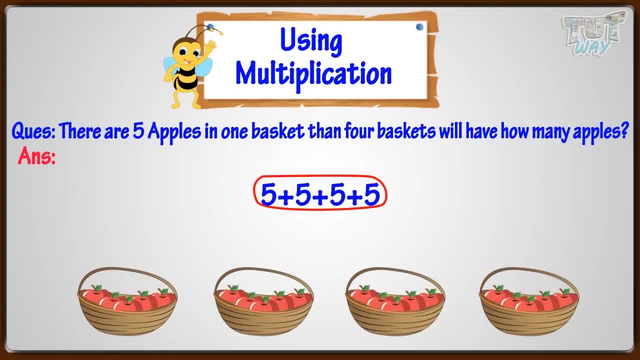 Plus 5 can be written as 5 times 4. And we can easily solve it, as 5 multiplied by 4 equals 20.. So 20 apples will be there in 4 baskets. Let's move on to another question. 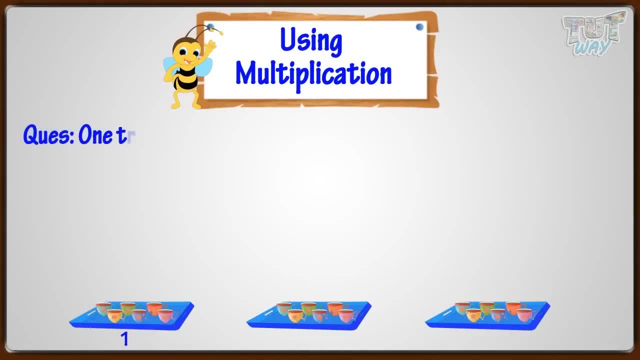 One tray holds 6 cups, Then 3 trays will hold how many cups. You need to add 6, 3 times here And you now know You can write repeated addition in the form of multiplication sentence. So adding 6, 3 times can be written as: 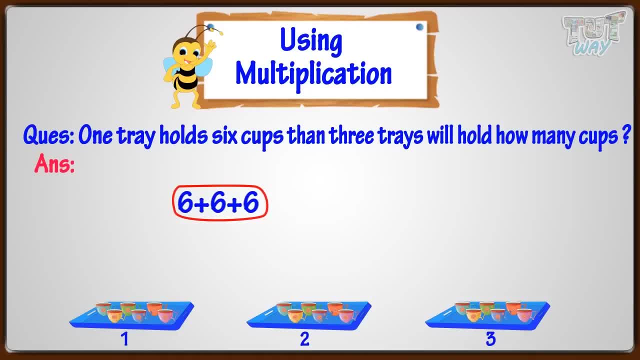 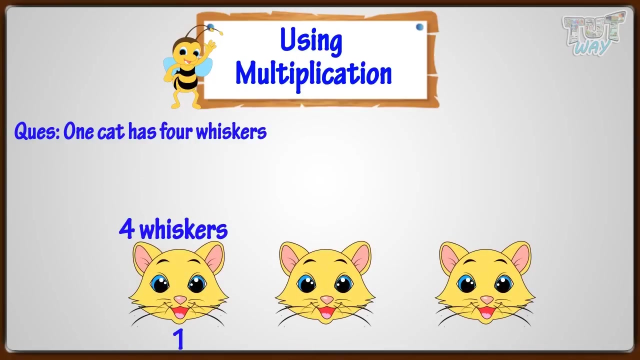 6 times 3.. And 6 multiplied with 3 is 18.. So 18 cups will be there in 3 trays. Let's move on to another question. One cat has 4 whiskers. Then 3 cats will have how many whiskers? 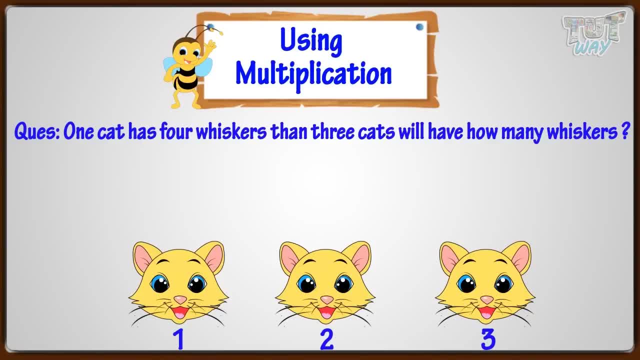 Then 3 cats will have how many whiskers? Then 3 cats will have how many whiskers We need to add the number of whiskers here. So it's a problem of repeated addition: 4 plus 4 plus 4.. 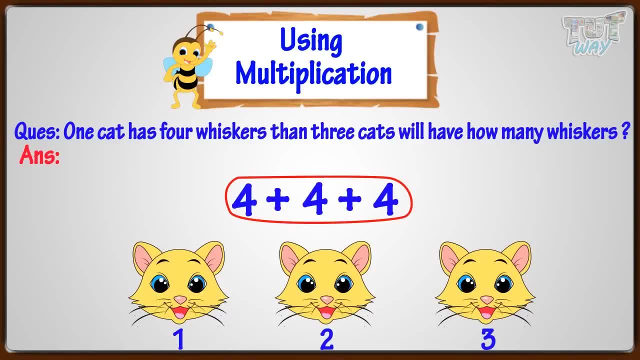 And we now know repeated addition problems- can be written as multiplication sentence. So we can write it as: 4 multiplied with 3. And 4 times 3 equals 12.. So 3 cats will have 12 whiskers. 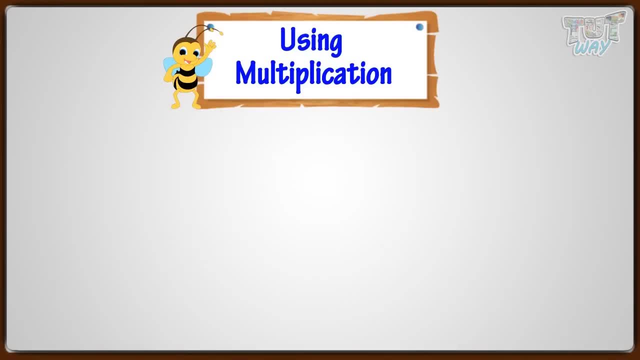 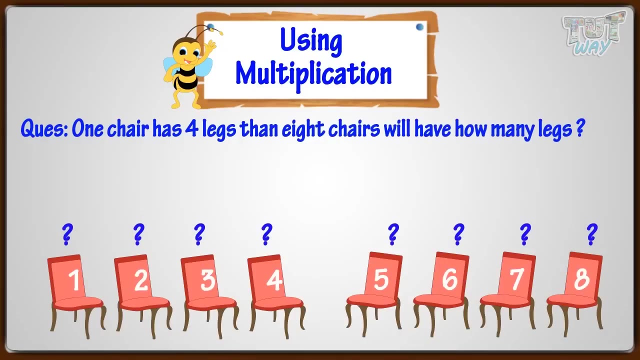 Now let's make one more multiplication sentence. One chair has 4 legs, Then 8 chairs will have. how many legs Can you make the multiplication sentence for this problem? Let's see We need to add the number of legs here. 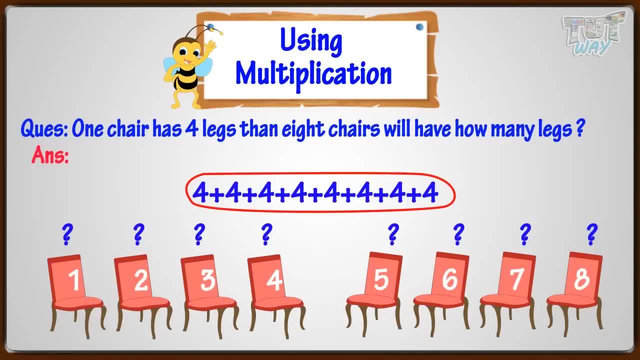 So it's a problem of repeated addition, Adding 4 8 times, So we can write it as 4 times 8.. So our multiplication sentence will be: 4 times 8 equals 32.. So our multiplication sentence will be: 4 times 8 equals 32..